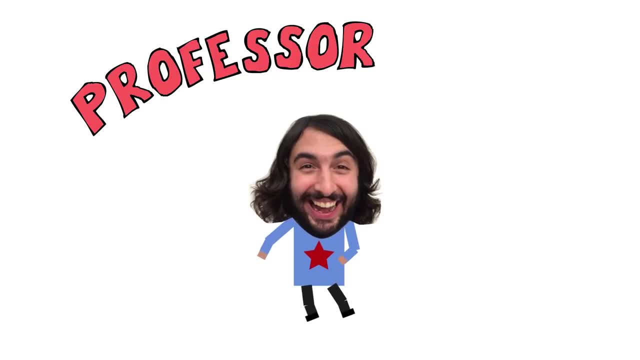 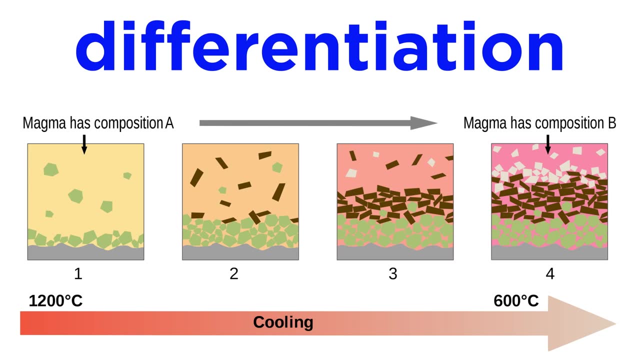 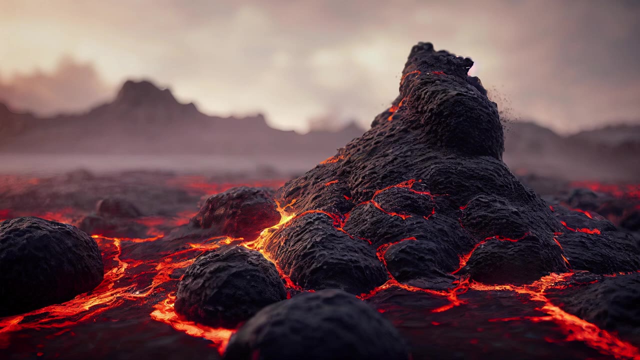 In the previous tutorial we learned about how rocks melt, differentiate and crystallize. Now we will discuss the different types of igneous rocks and how they are classified. Say you are given an igneous rock and asked what it is, Where would you begin? Your first step might? 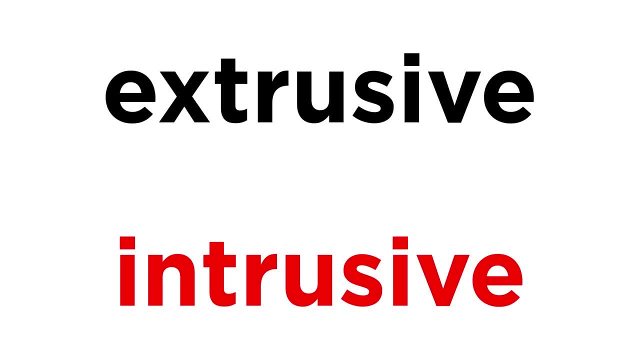 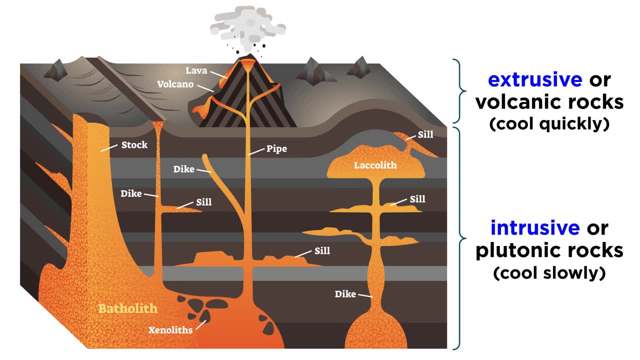 be determining whether it was extrusive or intrusive. Intrusive is a word describing an igneous rock that cooled slowly at depth, and extrusive is a word describing a rock that cooled quickly at the surface, usually during a volcanic eruption. Intrusive rocks are also called plutonic. 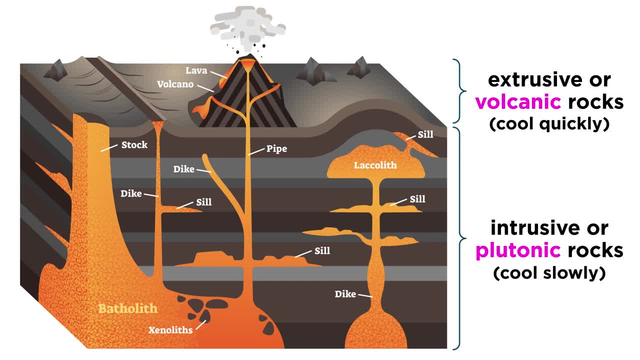 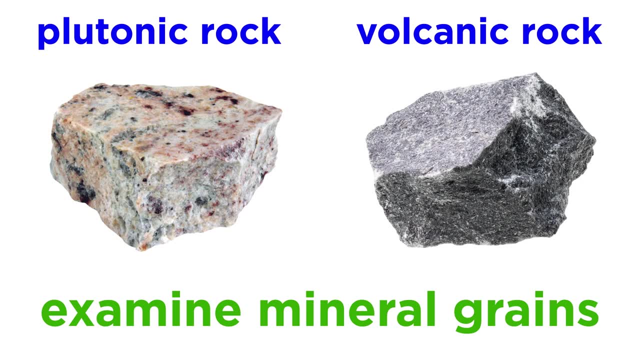 and extrusive rocks may be described as volcanic. It is usually pretty easy to distinguish a plutonic rock from a volcanic rock simply by analyzing the size of the mineral grains. Plutonic rocks, which cool slowly, have ample time to grow large crystals, while volcanic rocks 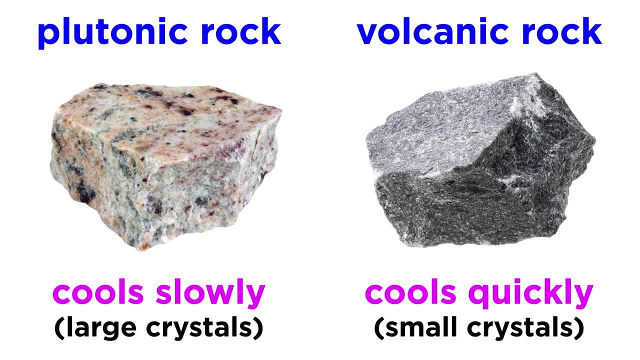 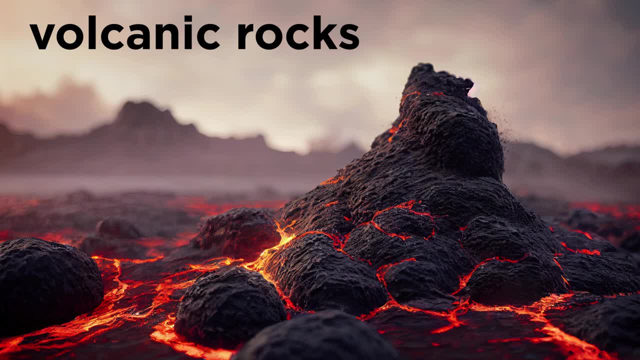 which crystallize rapidly, are composed of tiny grains that usually can't be seen by the naked eye. Let's first discuss volcanic rocks, since they are simply named after the magma from which they are derived. Both are classified based on their silica content and are as follows: 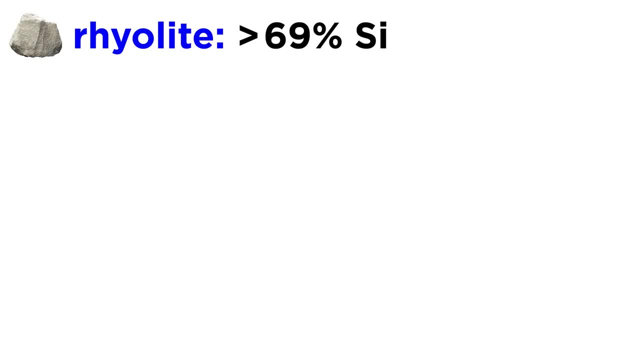 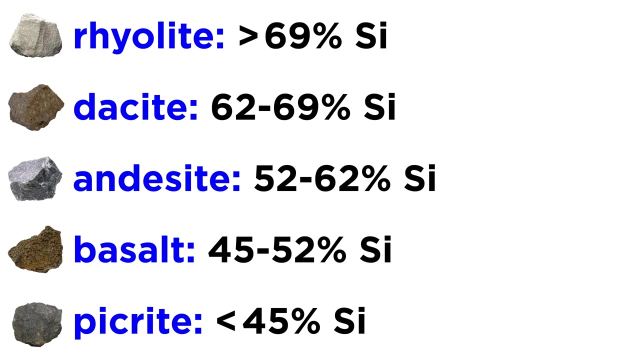 With rhyolite silica content is greater than 69%, dasite 62-69%, andesite 52-62%, basalt 45-52% and picrite, which contains less than 45% silica. The term ultramafic is commonly used. 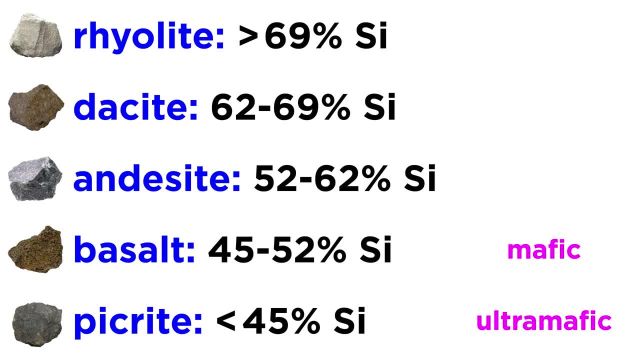 to describe picritic rocks, mafic for basaltic rocks, intermediate and intermediates, An idea mediate for andesitic rocks and felsic for dacitic and rhyolitic rocks. Rhyolite and basalt are very different rocks and it is typical for them not to have any. 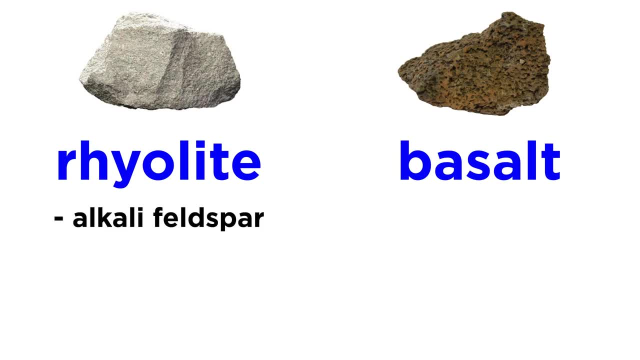 common minerals. For example, rhyolite is rich in alkali, feldspar, quartz and sodium-rich plagioclase with minor amounts of amphibole, while basalt is mainly composed of pyroxene olivine and. 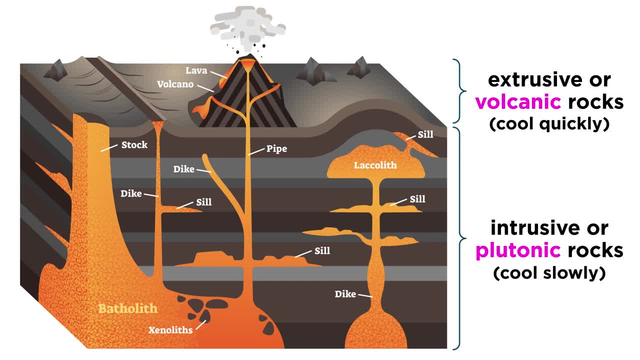 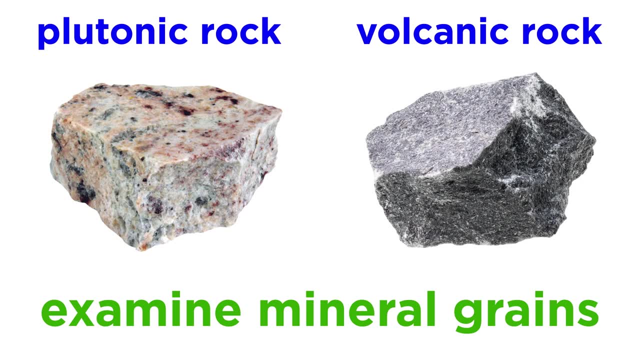 and extrusive rocks may be described as volcanic. It is usually pretty easy to distinguish a plutonic rock from a volcanic rock simply by analyzing the size of the mineral grains. Plutonic rocks, which cool slowly, have ample time to grow large crystals, while volcanic rocks 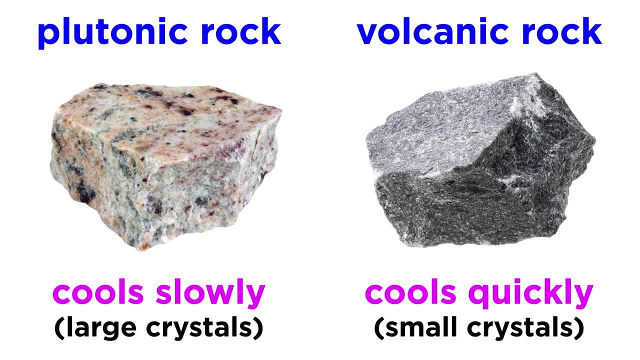 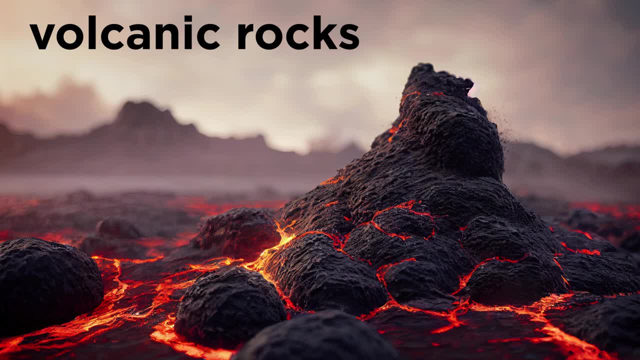 which crystallize rapidly, are composed of tiny grains that usually can't be seen by the naked eye. Let's first discuss volcanic rocks, since they are simply named after the magma from which they are derived. Both are classified based on their silica content and are as follows: 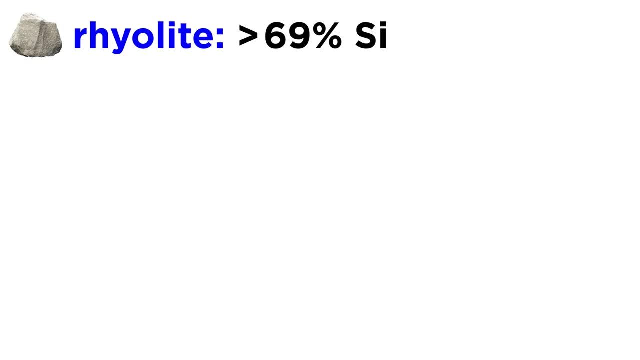 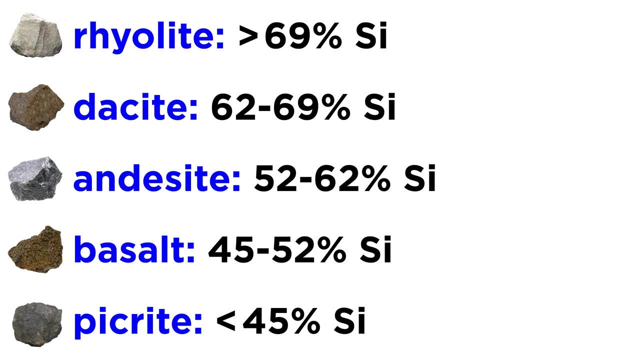 With rhyolite silica content is greater than 69%, dasite 62-69%, andesite 52-62%, basalt 45-52% and picrite, which contains less than 45% silica. The term ultramafic is commonly. 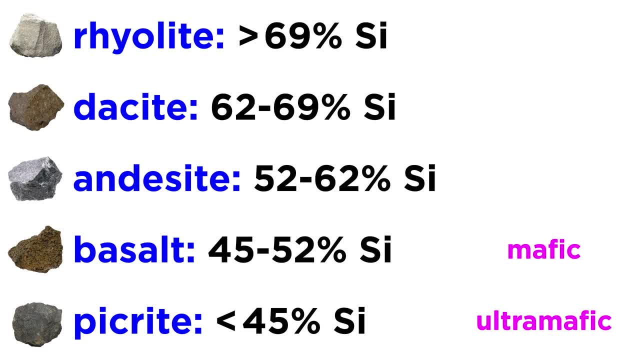 used to describe picritic rocks, mafic for basaltic rocks, intermediates for the entire, it for andesitic rocks and felsic for dacitic and rhyolitic rocks. Rhyolite and basalt are very different rocks and it is typical for them not to have any. 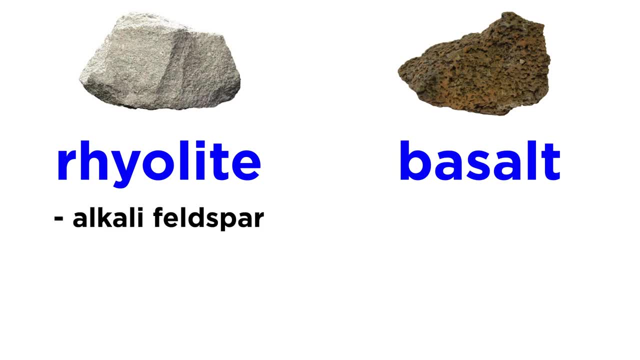 common minerals. For example, rhyolite is rich in alkali, feldspar, quartz and sodium-rich plagioclase with minor amounts of amphibole, while basalt is mainly composed of pyroxene olivine and. 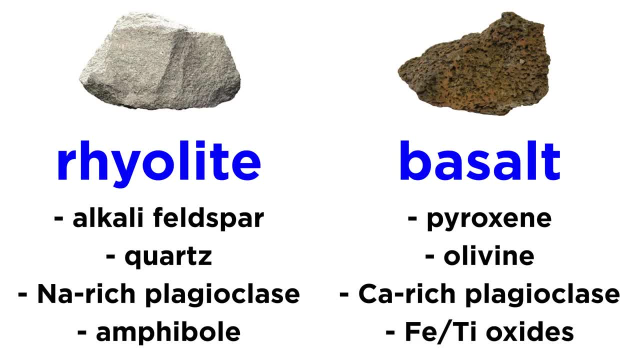 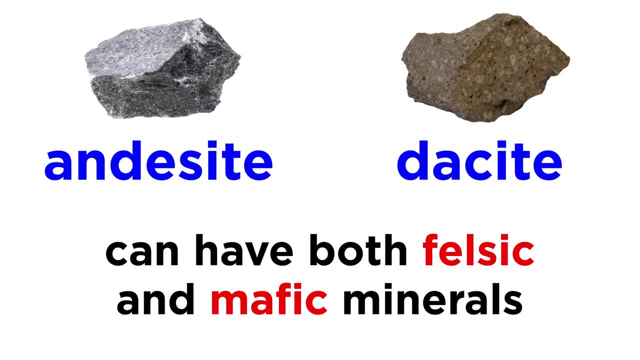 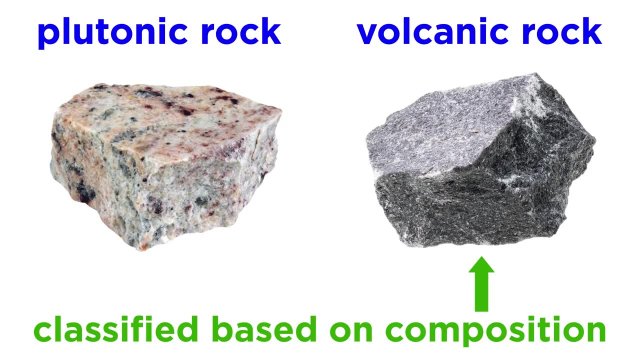 calcium-rich plagioclase with minor amounts of iron and titanium oxides. Andesites and dacites can have both felsic and mafic minerals, but are typically mostly plagioclase, with lesser amounts of pyroxene, amphibole and quartz. 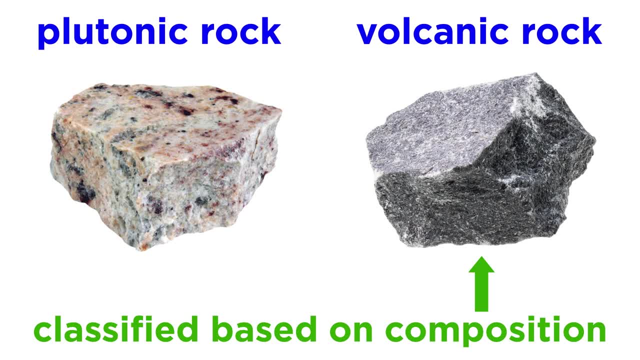 Plutonic igneous rocks have an entirely different naming convention than volcanic rocks, which are classified based on their composition, instead being named based on their three most abundant minerals. This is because the minerals in plutonic rocks can be easily identified in hand sample. 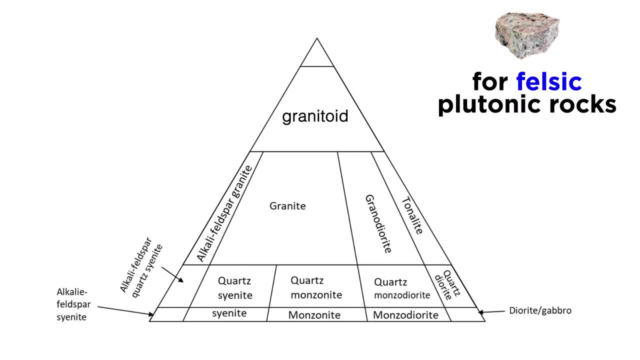 whereas volcanic minerals are typically too small For felsic-plutonic rocks. names are based on the relative amounts of quartz, plagioclase and alkali feldspar which are placed at the corners of a triangular or ternary diagram. 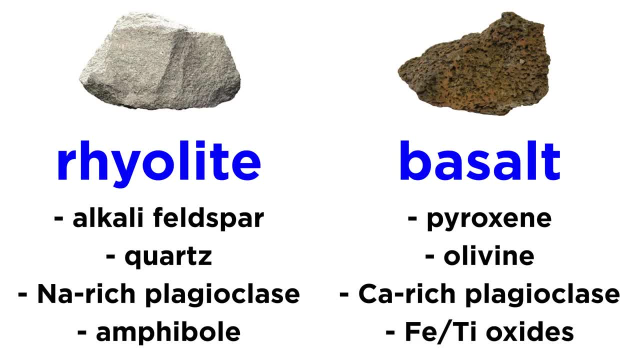 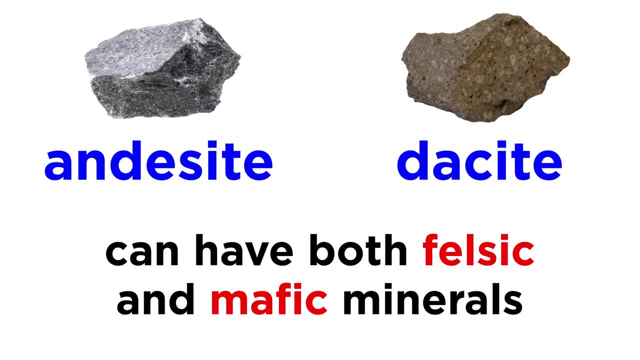 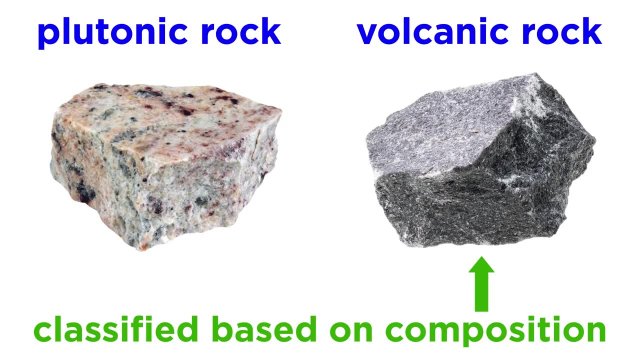 calcium-rich plagioclase with minor amounts of iron and titanium oxides. Andesites and dacites can have both felsic and mafic minerals, but are typically mostly plagioclase, with lesser amounts of pyroxene, amphibole and quartz. 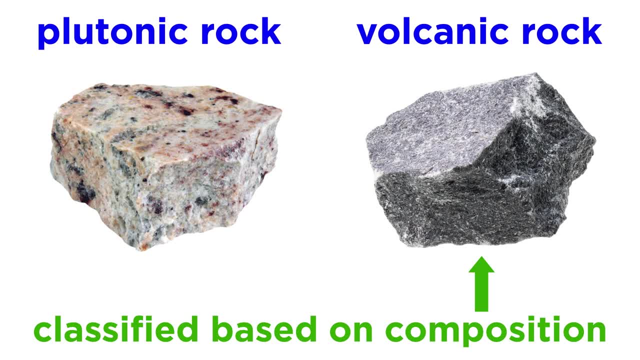 Plutonic igneous rocks have an entirely different naming convention than volcanic rocks, which are classified based on their composition, instead being named based on their three most abundant minerals. This is because the minerals in plutonic rocks can be easily identified in hand sample. 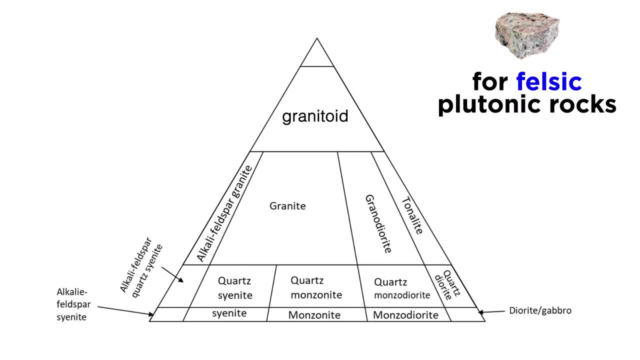 whereas volcanic minerals are typically too small For felsic-plutonic rocks. names are based on the relative amounts of quartz, plagioclase and alkali feldspar which are placed at the corners of a triangular or ternary diagram. 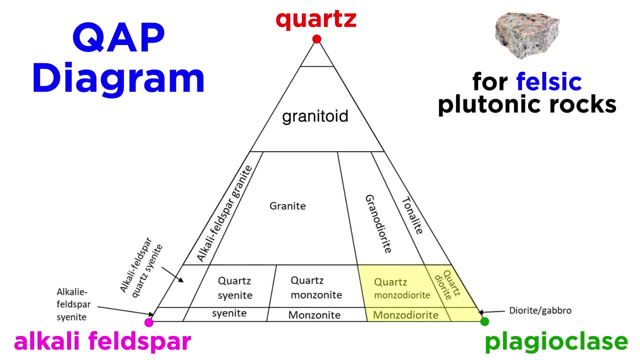 called a QAP diagram. Plagioclase-rich rocks are called diorite, Quartz-rich rocks are called granitoid Andesites and basalt are called diorites, And alkali feldspar-rich rocks are called cyanite. 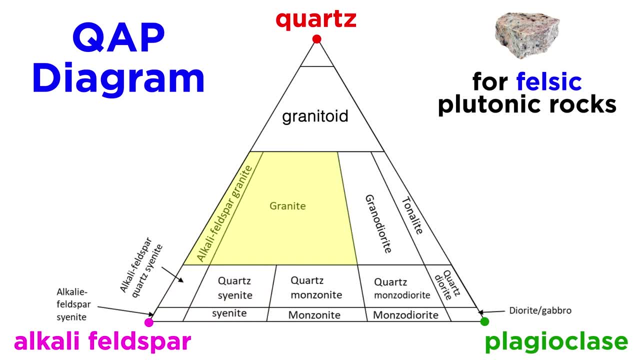 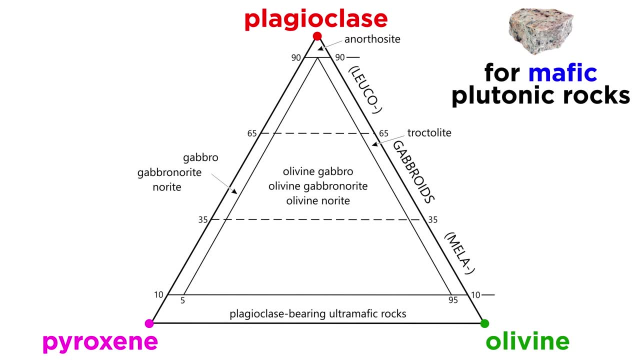 Rocks of intermediate composition are called granite if they are quartz-rich and manzanite if they are feldspar-rich. On the other hand, mafic-plutonic rocks are named based on their relative abundances of olivine, pyroxene and plagioclase and again are plotted on ternary diagrams. 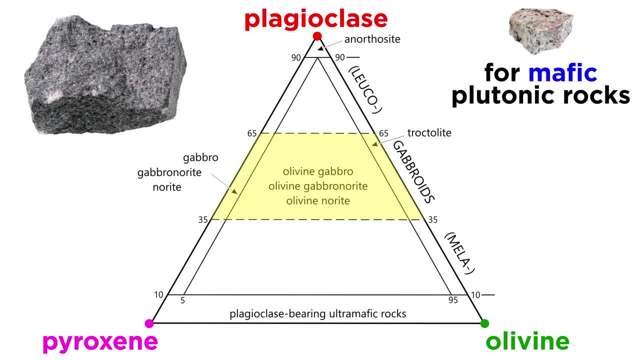 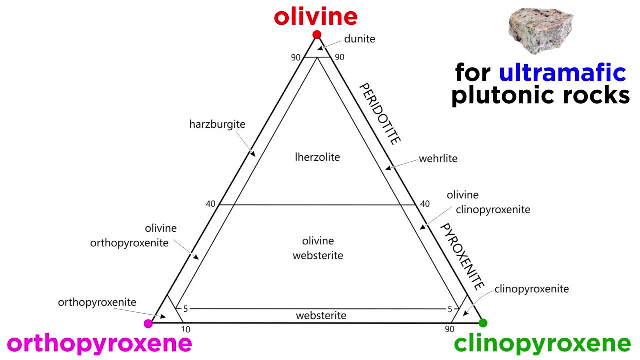 Gabbro, which is the plutonic version of basalt, contains roughly equal parts plagioclase and clinopyroxene. Likewise, ultramafic rocks can be classified using the minerals olivine, clinopyroxene and orthopyroxene. 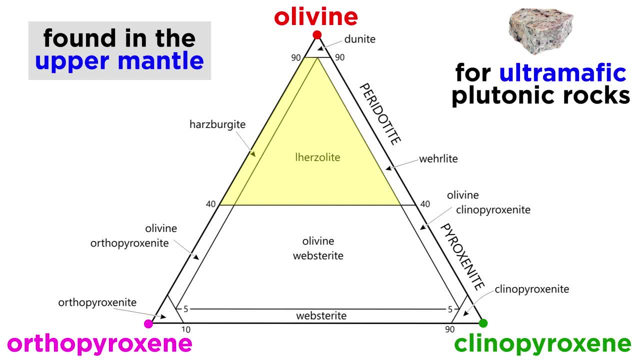 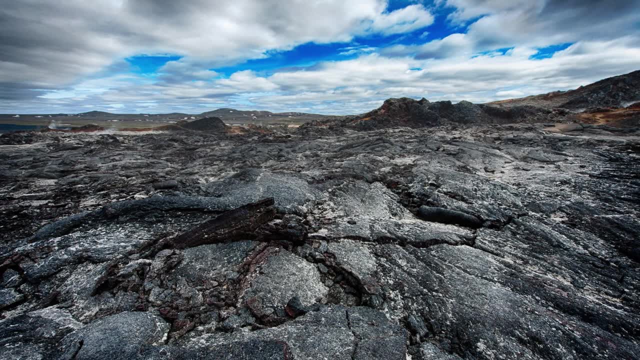 These rocks, like harzbergite and lairzolite, are representative of the upper mantle and are rarely found at the surface. So what types of igneous rocks are found at the surface? That depends on where you look. For instance, the lava that erupts from mid-ocean ridges is exclusively found at the surface. 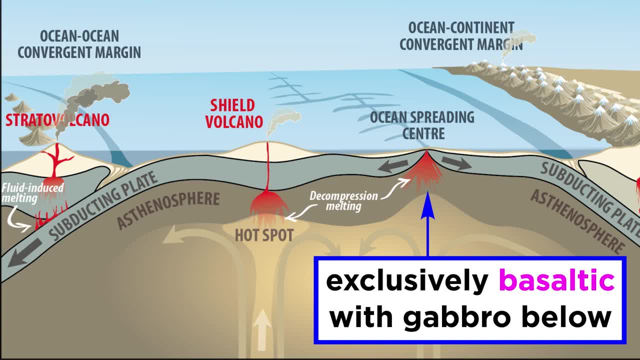 The lava that erupts from mid-ocean ridges is exclusively found at the surface. So what types of igneous rocks are found at the surface? That depends on where you look. So what types of igneous rocks are found at the surface? 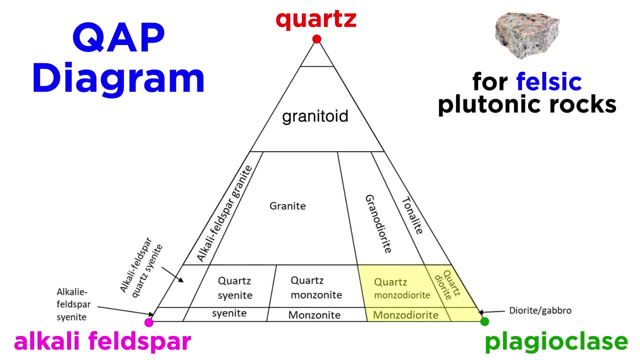 called a QAP diagram. Plagioclase-rich rocks are called diorite, Quartz-rich rocks are called granitoid Andesites and basalt are called diorites, And alkali feldspar-rich rocks are called cyanite. 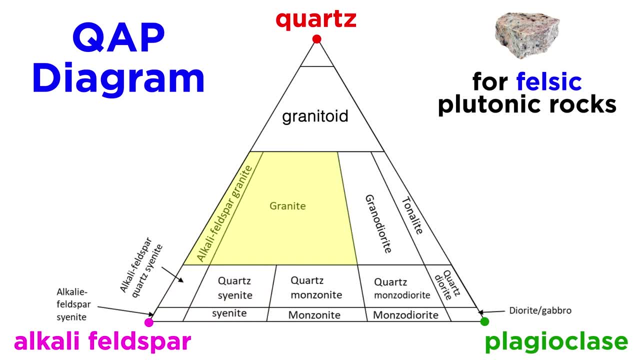 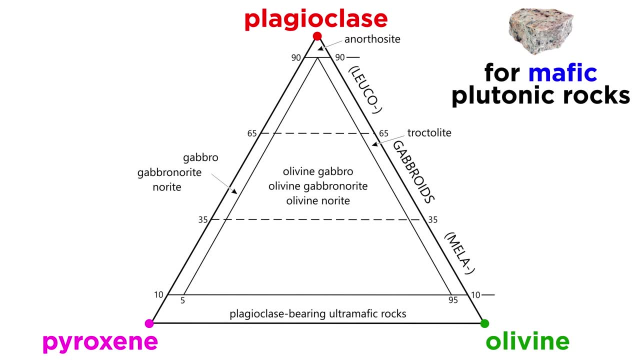 Rocks of intermediate composition are called granite if they are quartz-rich and manzanite if they are feldspar-rich. On the other hand, mafic-plutonic rocks are named based on their relative abundances of olivine, pyroxene and plagioclase and again are plotted on ternary diagrams. 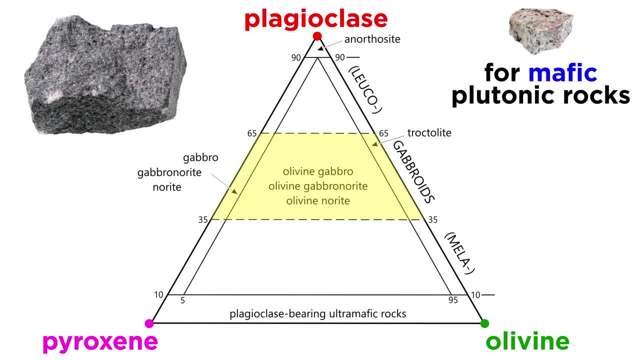 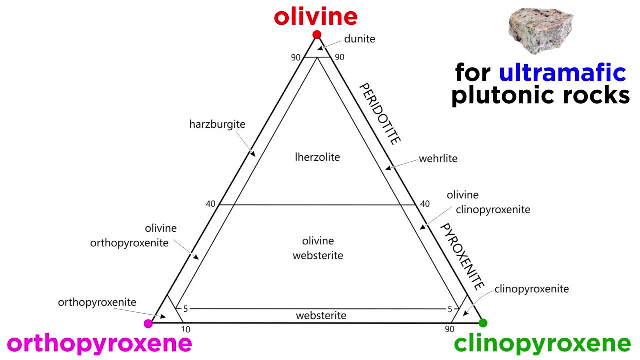 Gabbro, which is the plutonic version of basalt, contains roughly equal parts plagioclase and clinopyroxene. Likewise, ultramafic rocks can be classified using the minerals olivine, clinopyroxene and orthopyroxene. 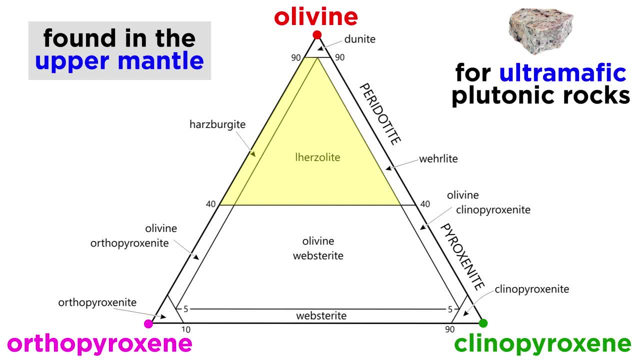 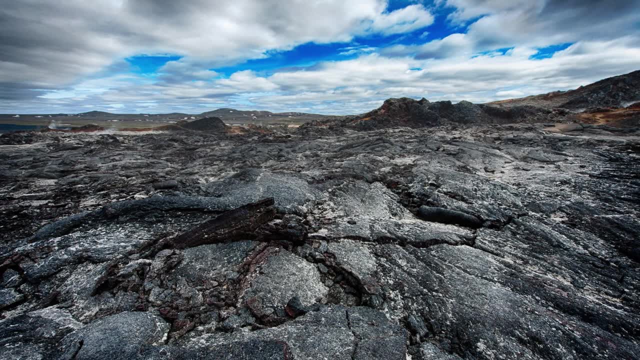 These rocks, like harzbergite and lairzolite, are representative of the upper mantle and are rarely found at the surface. So what types of igneous rocks are found at the surface? That depends on where you look. For instance, the lava that erupts from mid-ocean ridges is exclusively found at the surface. 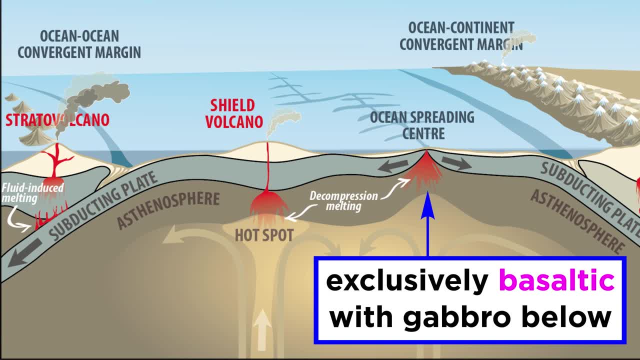 The lava that erupts from mid-ocean ridges is exclusively found at the surface. So what types of igneous rocks are found at the surface? That depends on where you look. So what types of igneous rocks are found at the surface? 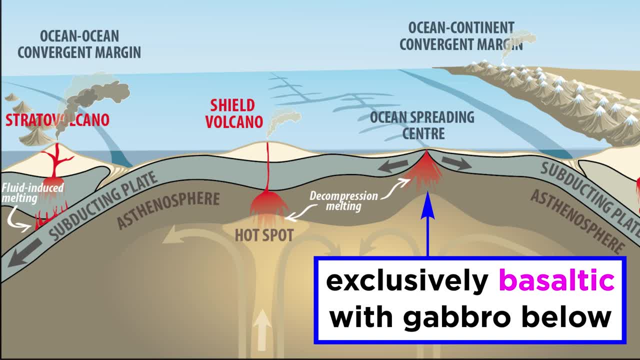 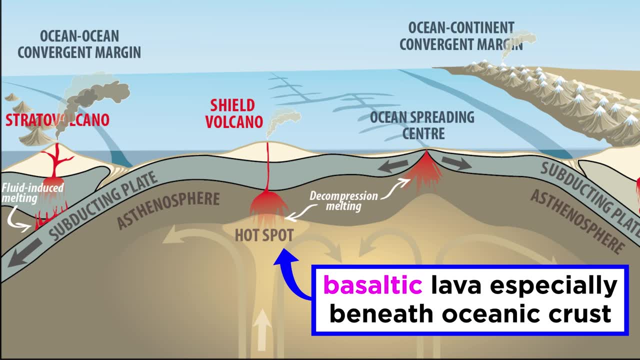 The lava that erupts from mid-ocean ridges is exclusively basaltic, with gabbro forming deeper beneath the surface, which is basically just basalt with big crystals. Hotspots are also capable of producing massive amounts of basaltic lava, especially when 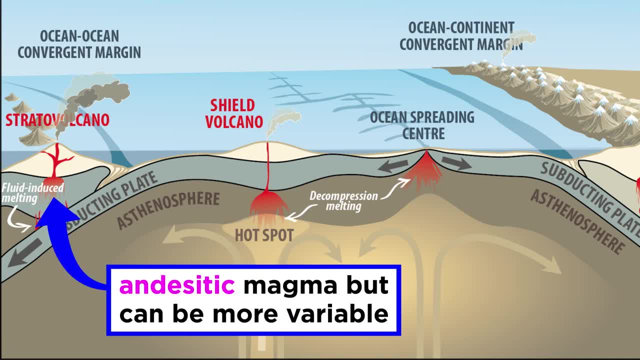 they are beneath oceanic crust. Subduction zones tend to produce andesitic magma but can be much more variable, also being influenced by crustal thickness Island arcs, which are subduction zones where the overriding plate is oceanic crust are. 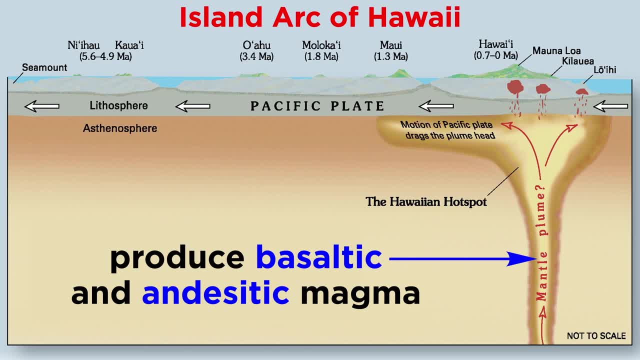 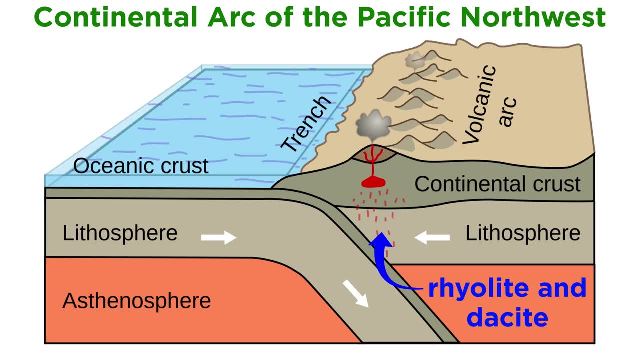 tend to produce basaltic and andesitic magma, while continental arcs like the volcanoes of the Pacific Northwest tend to erupt, rhyolite and desite With igneous rocks now covered, let's move forward and check out some other types of.